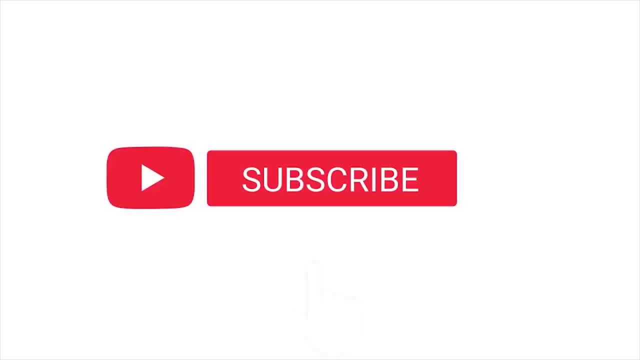 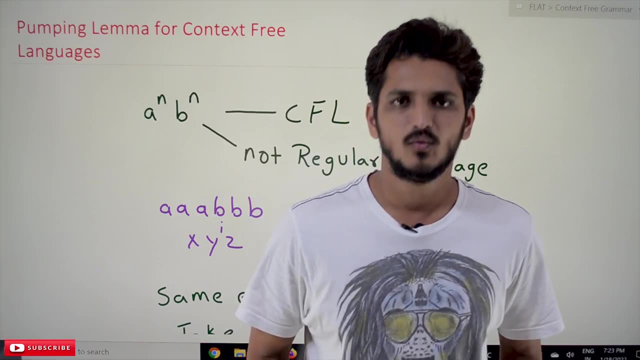 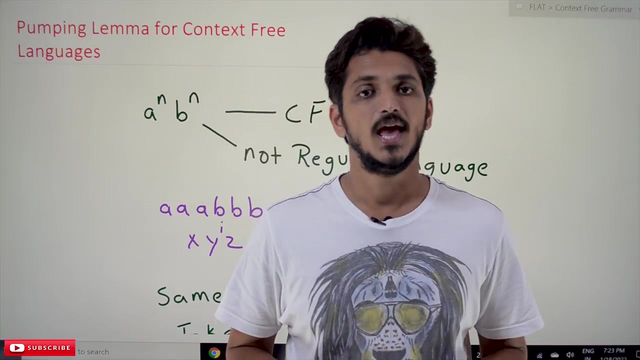 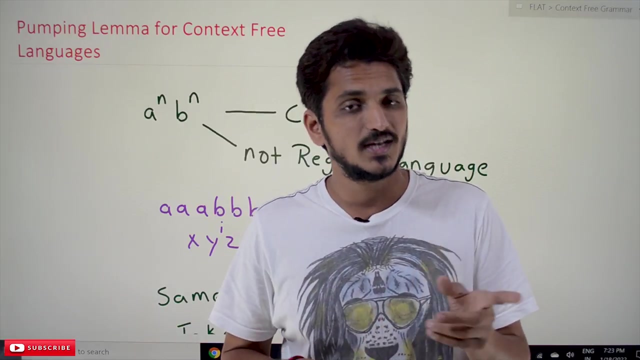 Hi, welcome to Learning Monkey. I am Raghu here In this class we will discuss about pumping lemma for context-free languages. In our previous classes we already discussed about the failure case of context-free languages and we already discussed about pumping lemma for regular. 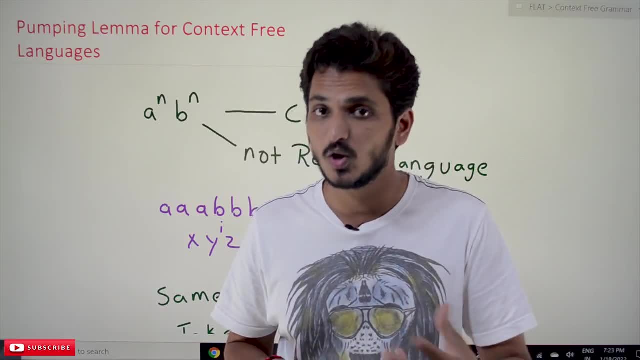 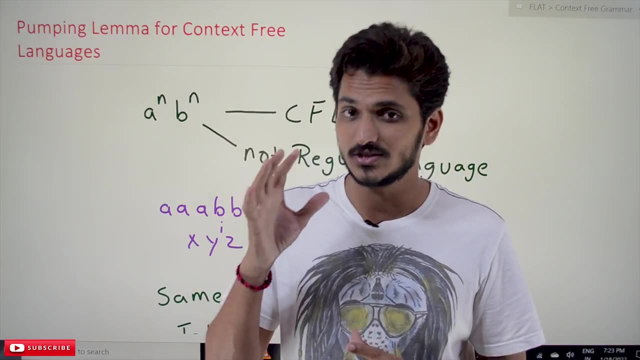 languages. Please watch those classes and come back here. They will help you a lot in understanding this class. The link for the playlist is provided in the description below. Coming to today's class, let's refresh the concept of pumping lemma for regular languages. 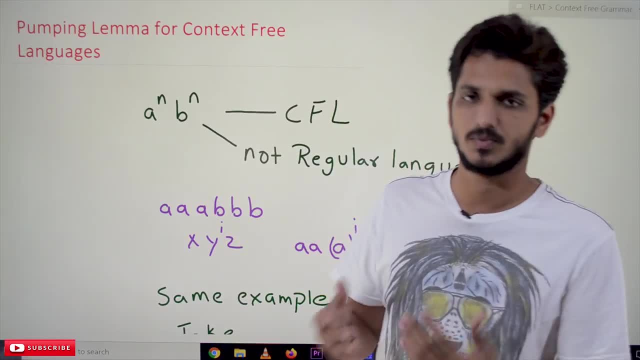 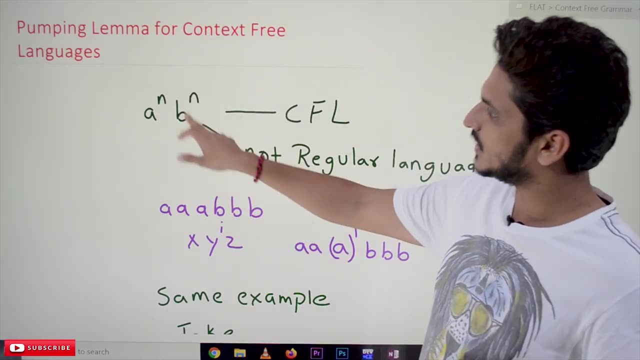 Along with that we will come into the concept of context-free languages, pumping lemma for context-free languages. So this is the example for context-free languages: A power N. B power N. It is a context-free language, but it is not a regular language We discussed 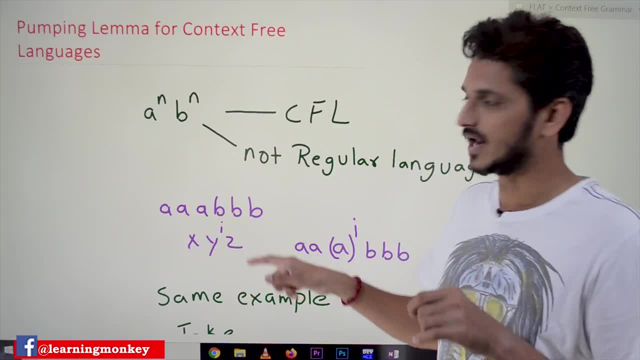 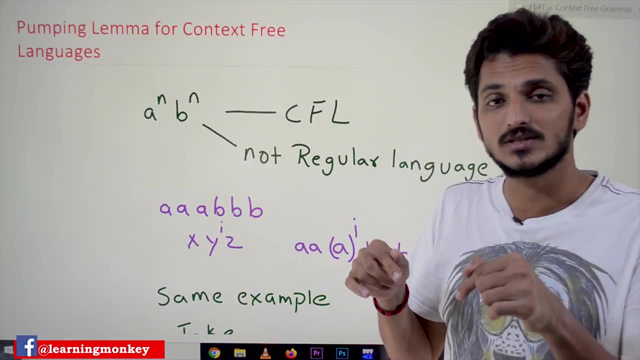 it in the previous class. So let's get started. It is not a regular language. Why it is not a regular language? What's the strings that are present here? A is followed by equal number of Bs In regular languages. we cannot do. 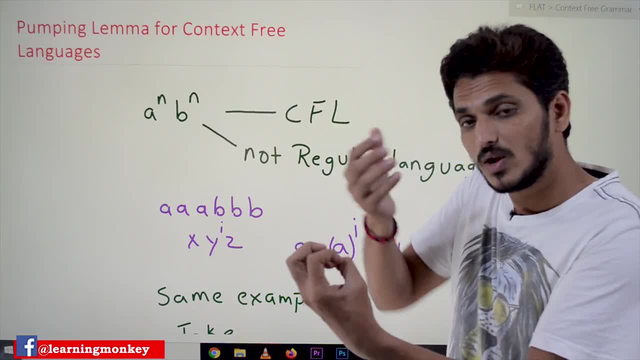 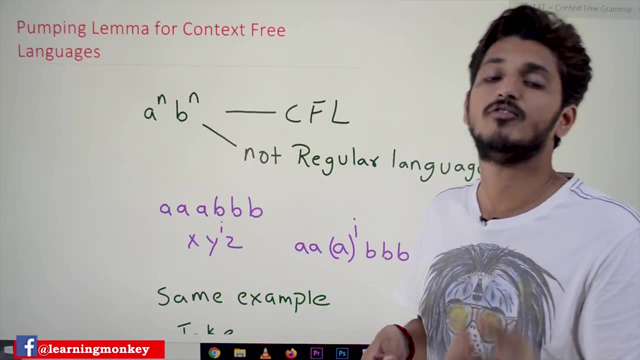 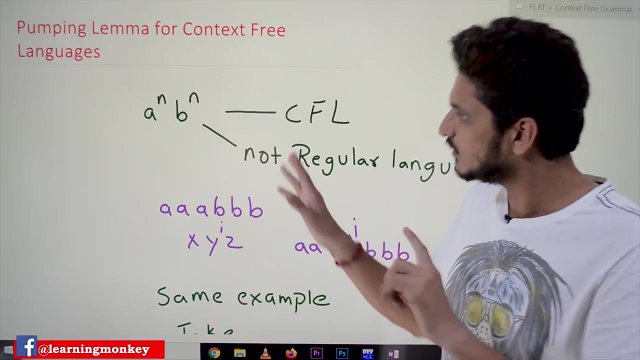 the equality count A is followed by equal number of Bs. We cannot do the counting equality check Why? We don't have a memory in a finite automata. That's why we cannot check. But in context-free languages we had a memory, stack memory. That's why we can check. 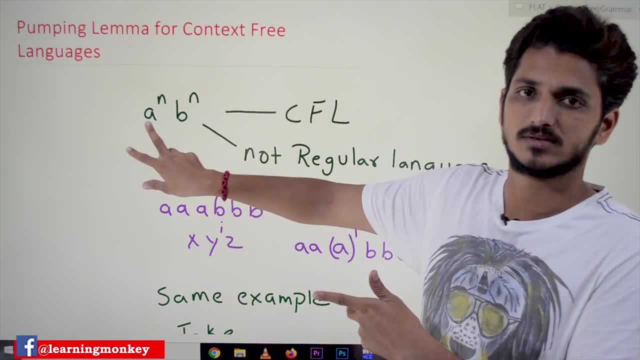 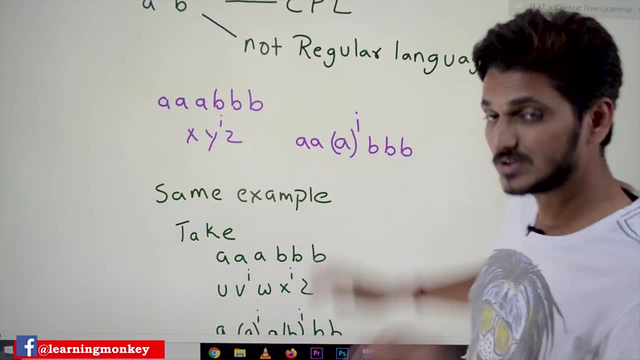 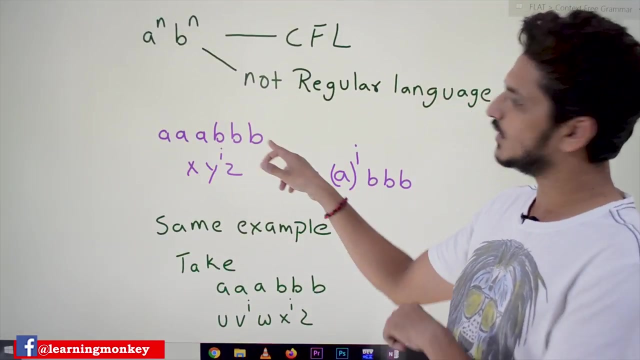 The count equality check for two symbols. This point we discussed in our last class, So based on that. so what's the pumping lemma for regular languages? we have done A, A, A, B, B, B. This is the language. A is followed by equal number of Bs. We divide this input. 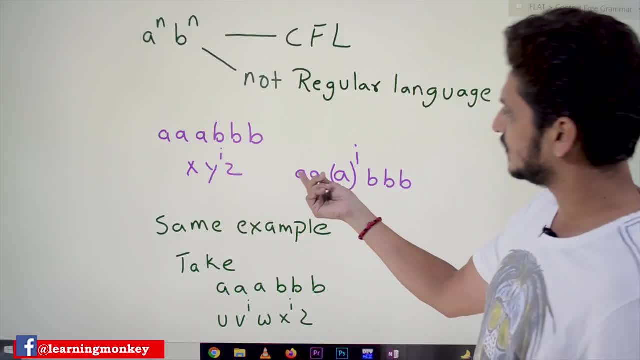 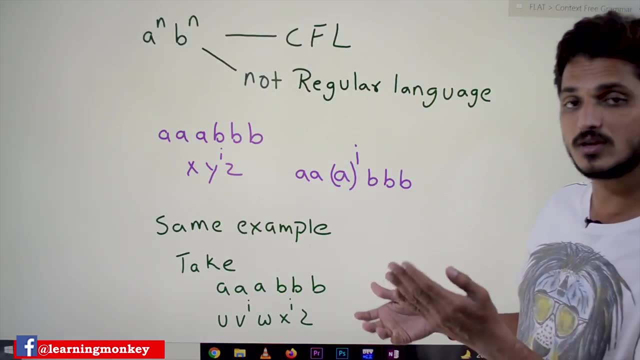 string into three parts: X, Y, power I, Z. We divided it to X as A, A, A, power I. We keep on pumping this A. So if you keep on pumping this A, you will get the same number of Bs. If you got the strings that are present in the language, it is a regular language. 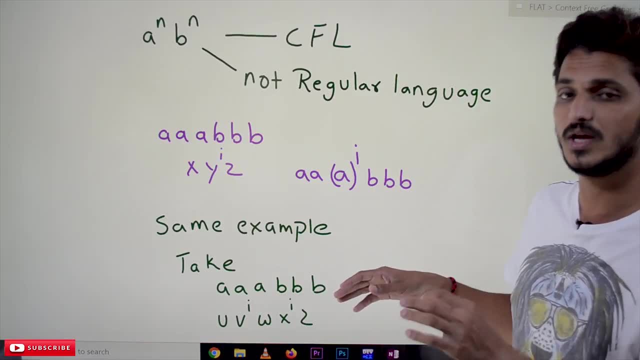 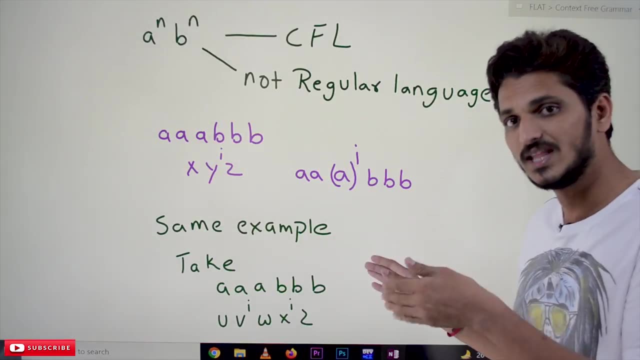 Otherwise, if you check for all the possibilities and prove that we are not going to get the strings that are present in the language, we say that the language is not in the regular language. That is what the logic we discussed when we discussed about pumping lemma for. 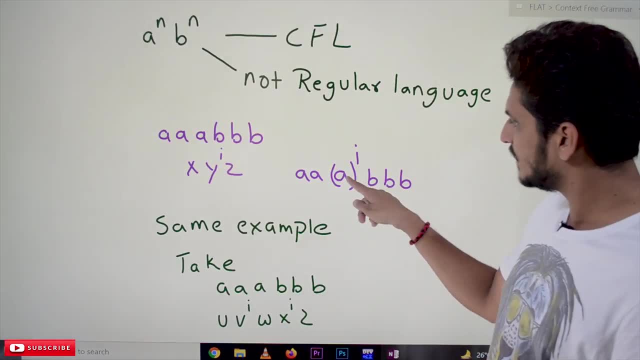 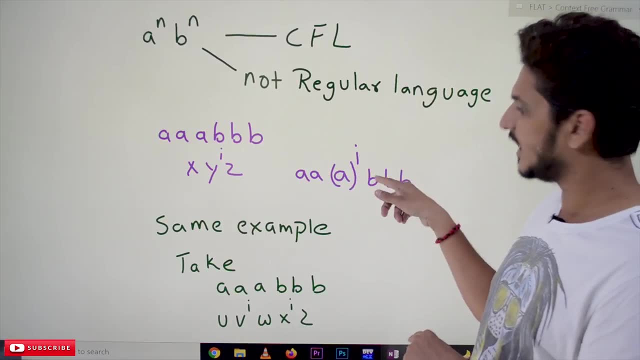 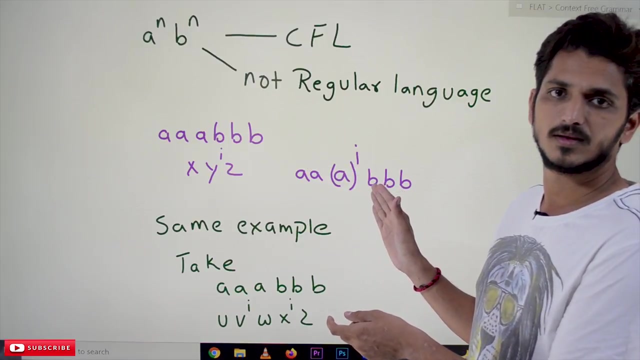 regular languages. See here we will understand this: A power I: If you keep on pumping A power one, it means A, A, A, B, B, B. A power two: A, A, A, A, B, B, B. We keep on pumping A, but we are not keep on pumping B, So that 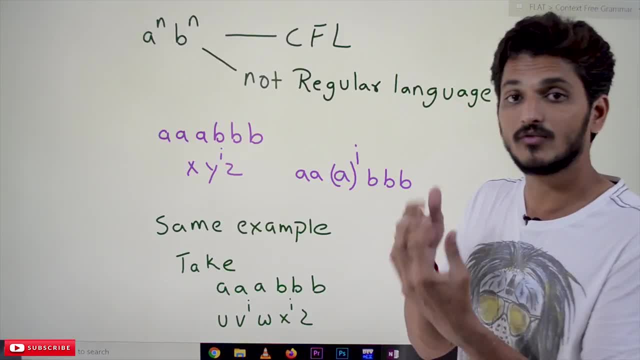 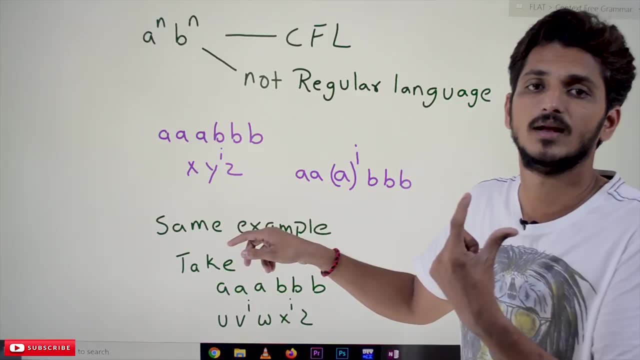 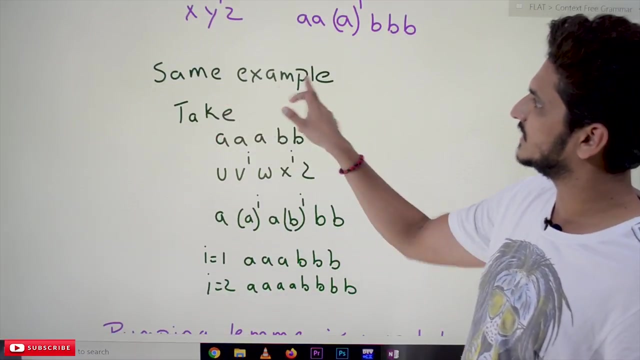 is why regular languages can't do the count. Count of equality check for two symbols. That is why we have taken only single pumping variable. But coming to context, free languages: see here For the same example. if you take an example like this, Same example: A, A, A. 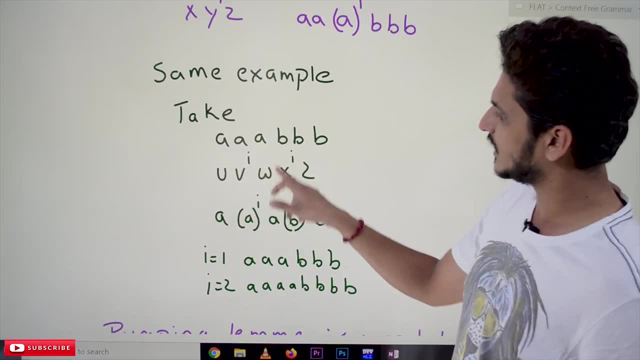 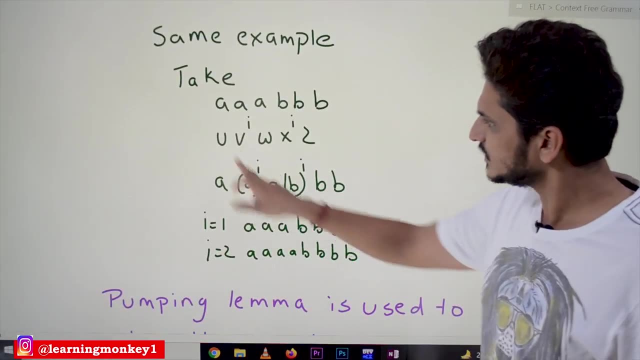 B, B, B. If you divide the string into five parts you will get the same number of Bs, So you have five parts. U, V, power I, W, X. power I Z means we are taking two pumping variables. See what happens now: U as A, V as A. A. power I means pumping variable W. 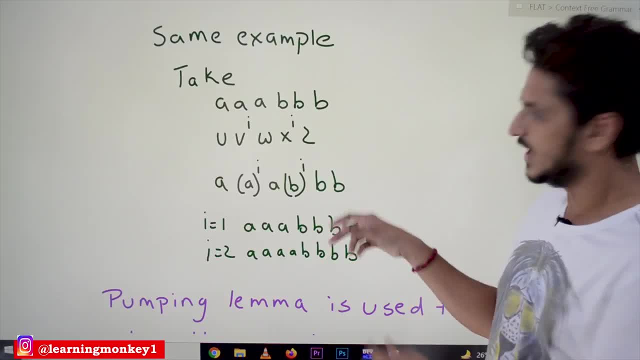 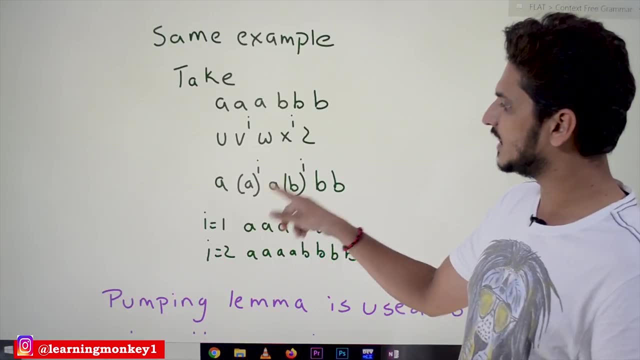 as A, X as B and Z as B B. If you keep on pumping, I? I is equal to one. we will get A, A, A, B, B. B I is equal to two. we will get A, A, A, A, B, B. B B Means we are getting. 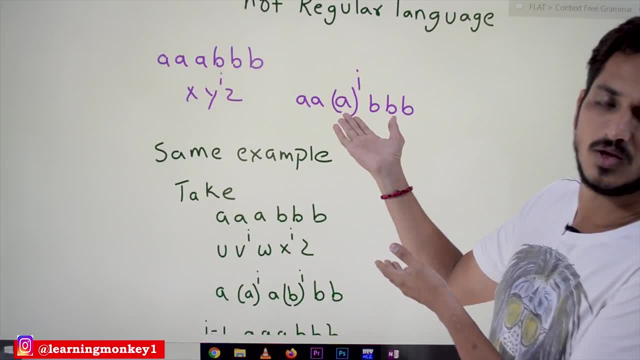 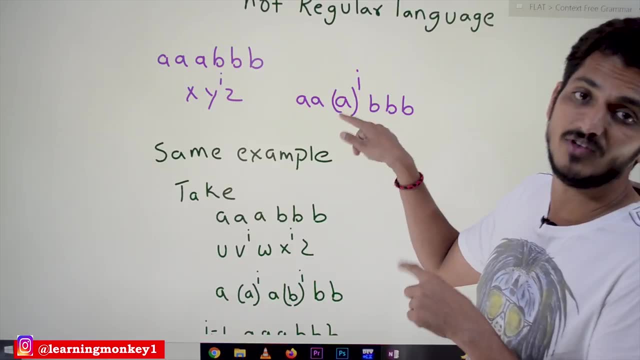 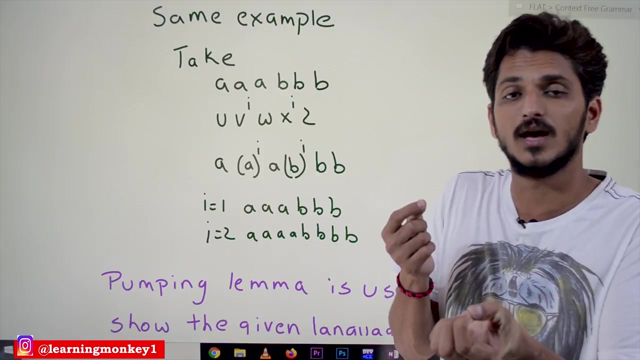 if you take two variables here, this won't work. We cannot prove that this language is not belonging to regular language. That's why we have taken only single variable here. If you take two variables, two pumping variables, we can do equality check for two symbols, But context: free languages If you want to. 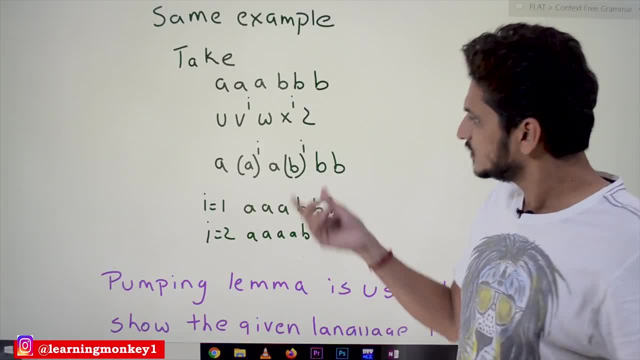 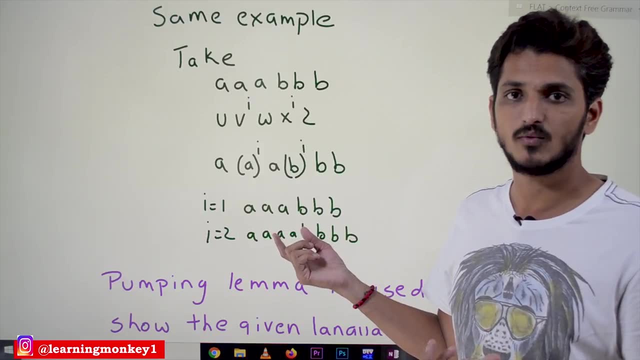 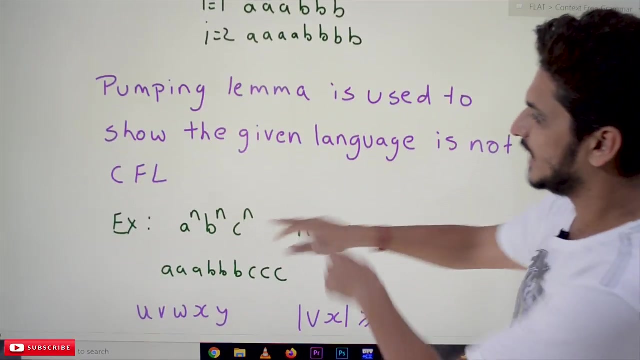 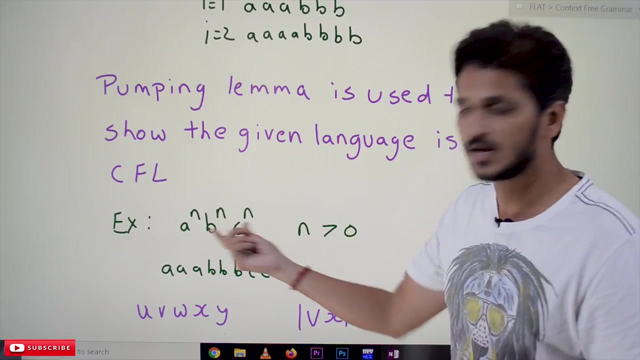 show that the given language is not context free language. so two variables are not enough. You understand that why? why two variables are not enough? the example which is not context free language is pumping is a power n, b power n and c power n means you need equality of three variable count, three symbol count. 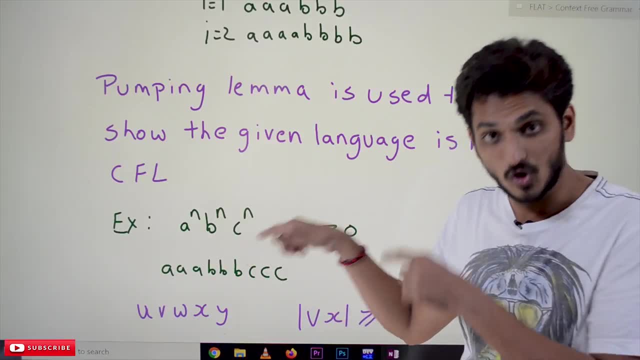 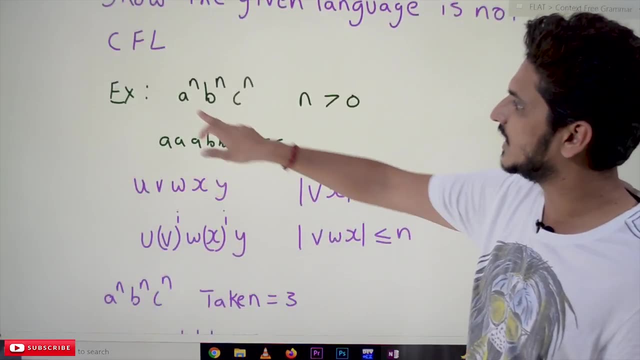 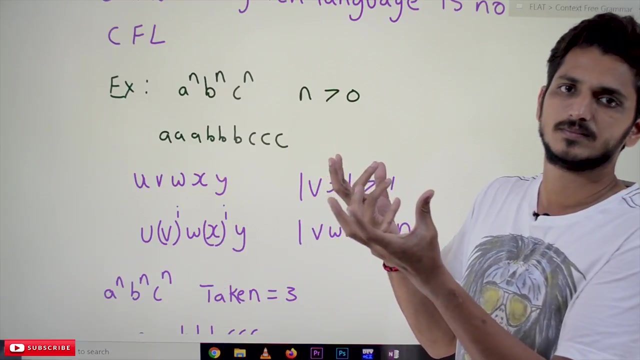 here. this is not a context free language. that's why we have chosen, in the context free language, we have chosen that we will divide a power n, b power n, c power n. we will divide that into five parts and two parts going to pump. okay, that is what the essence of a pumping lemma for context. 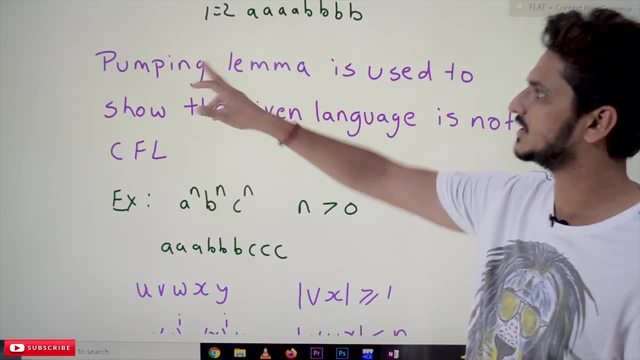 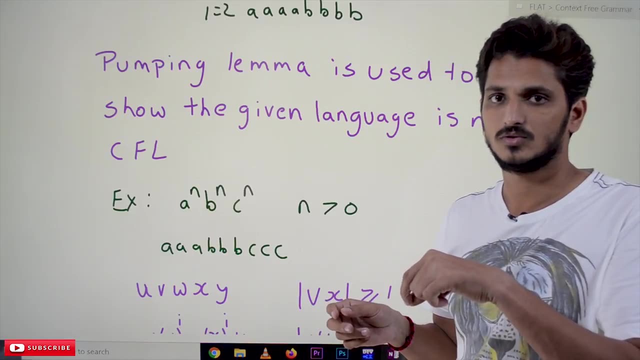 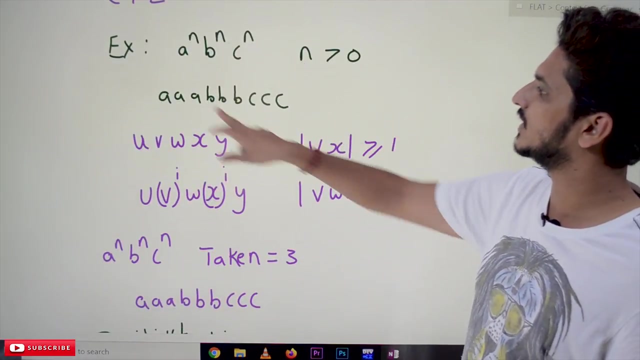 free languages now coming to come pumping lemma for context free languages. pumping lemma is used to show that the given language is not context free language. so it is going to show the given language is not context free language. so how to show that? a power n, b, power n, c, power n we. 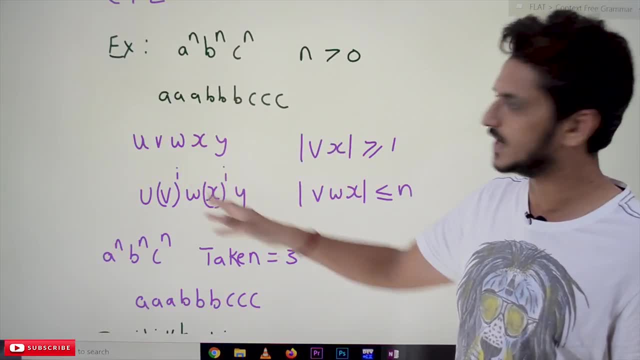 this is the input string we have taken, divided into five parts: u, v, d and c. power n. this is the input string we have taken, divided into five parts: u, v, d and c. power n, w, x, y, u is taken as u. you check all the possibilities and each possibility if you. 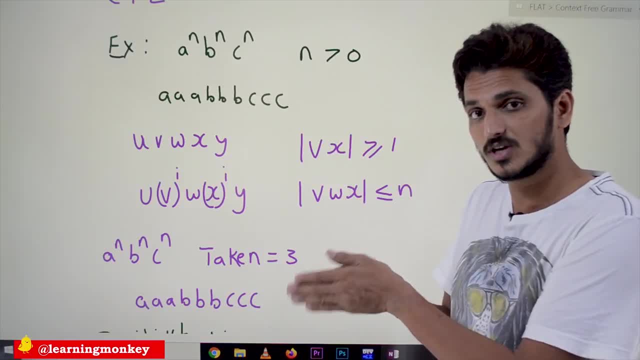 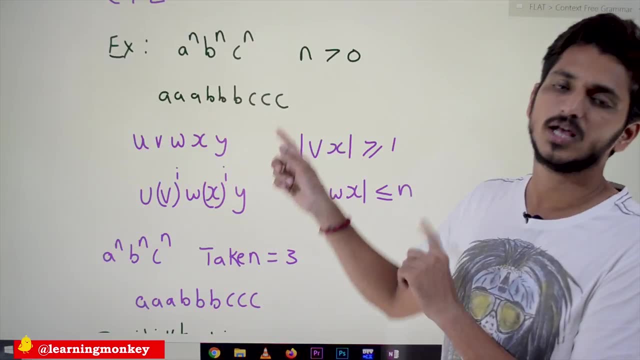 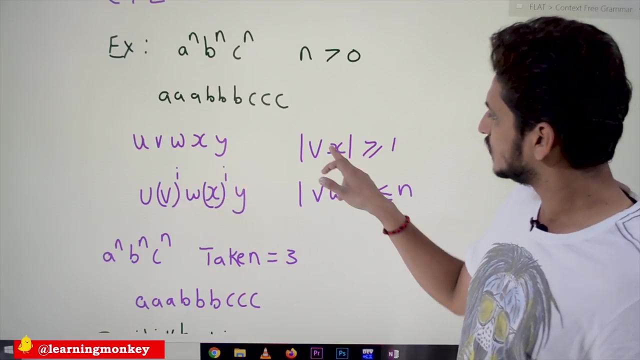 show that this is not going to generate the strings that are present in the language. if you show it, for all the possibilities, yes, we can say that the given language is not a context free language and we have to follow these conditions. we are going to pump v power i, x power, i, so that's. 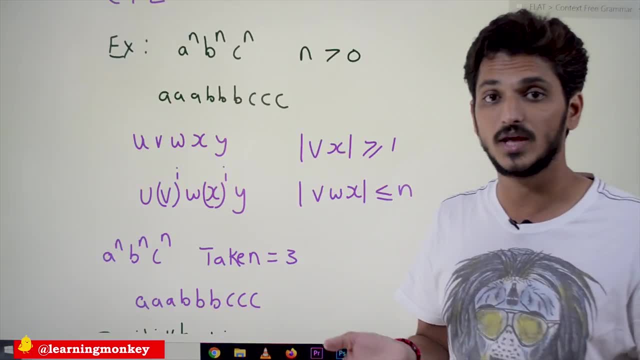 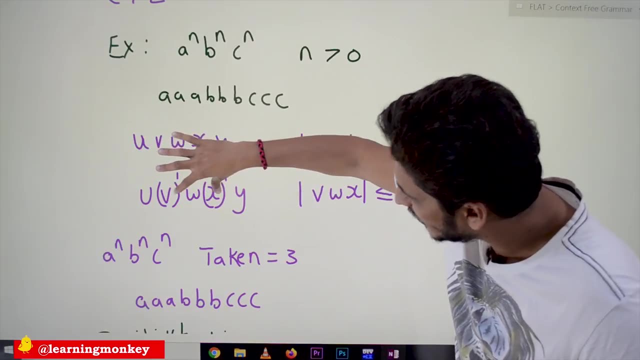 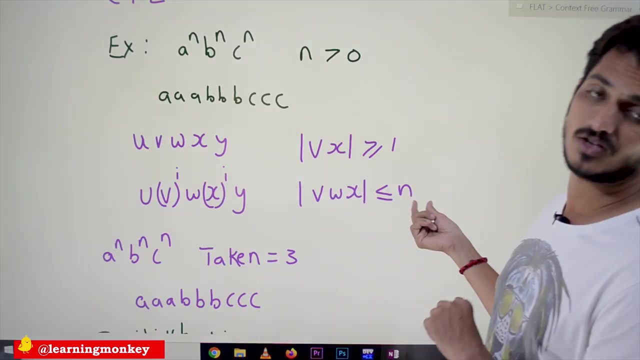 why v x should be greater than or equal to one. you are not supposed to take v x as epsilons. there is no use of that. that is the condition it is saying, and the middle part, v w x, the- whatever the possibility we consider here, v w x. so this should not be less than or equal to n. this should. 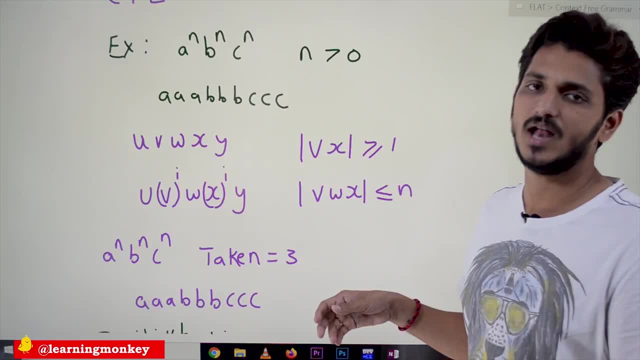 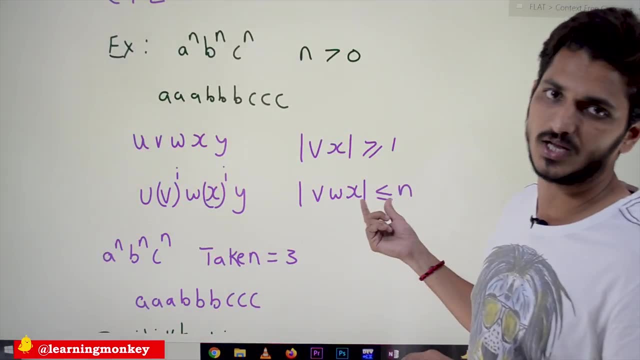 be less than or equal to n. what is this n? you can take any n value. in order to make the string as short as possible and to check all the possibilities, this n has been chosen. let's try to understand with an example. if you take that a power, n b power and c power and take n is equal to three. 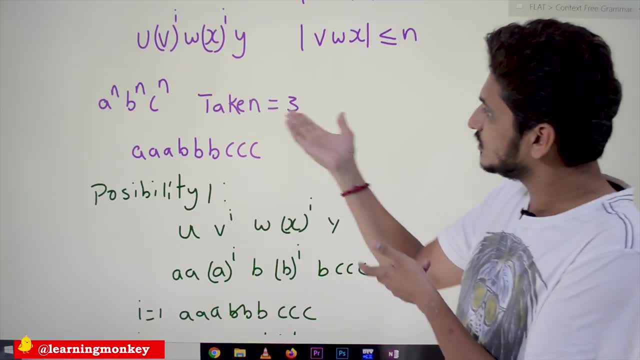 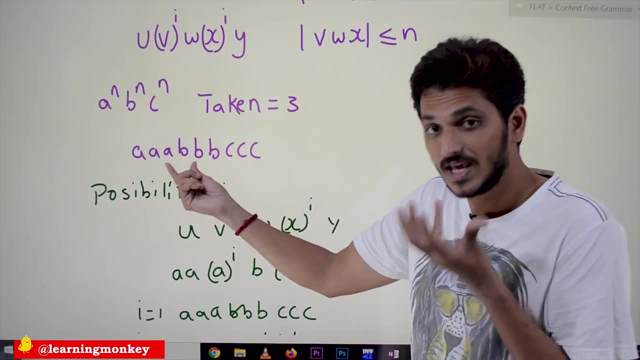 so you can take any n value and you can take any n value and you can take any n value and you can. this is the input string, possibility 1. so whenever you take that n is equal to 3, the middle part VWX, you can choose only these three A's means only A's. 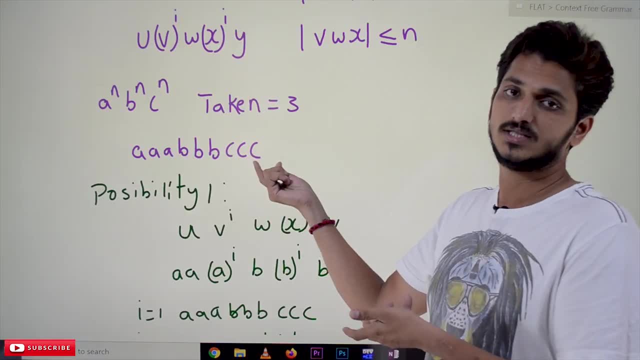 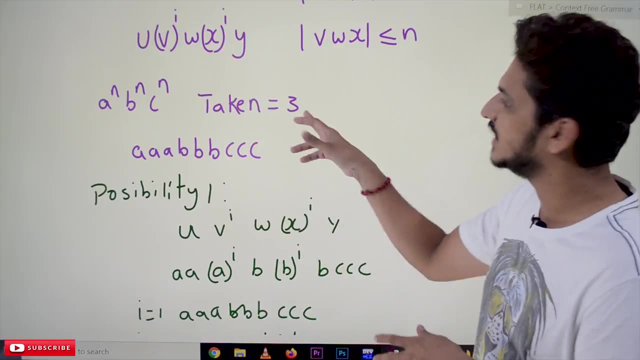 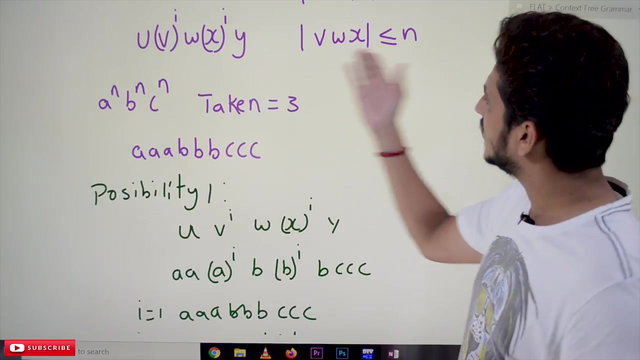 possibilities, only B's possibilities, only C's possibilities, combination of A- B possibilities, combination of B- C possibilities- all are possible with this n value. that is enough to show that the given language is not context free language. so that's why you can take any n. so now we will show two possibilities. 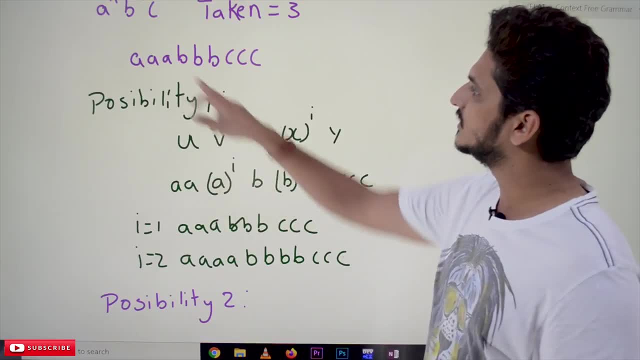 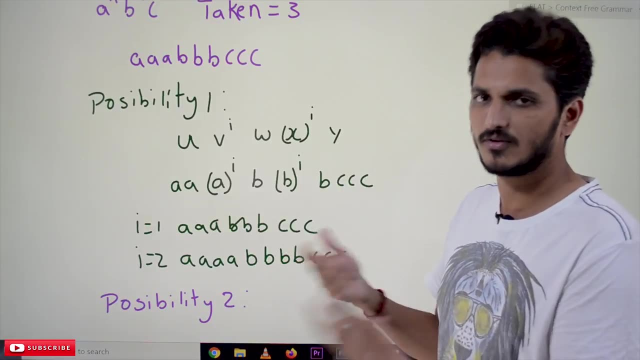 like that. you have to show all the possibilities. possibility 1: if you take this A, A, A, B, B, B, C, C, C, U, V power I, W, X power I- it's not X power, we are in the flow, we are talking it as X power I. we keep some pump the X variable, Y. so if 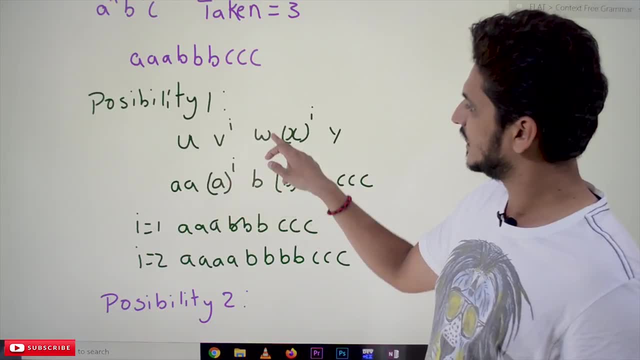 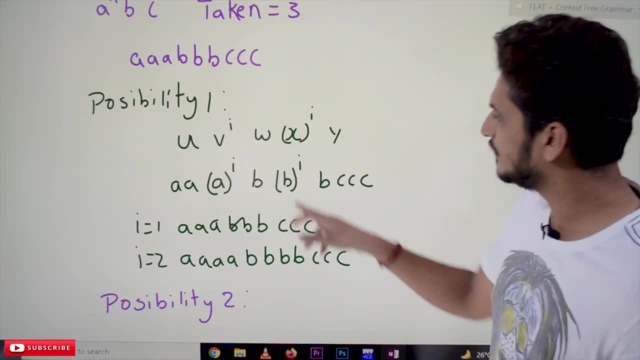 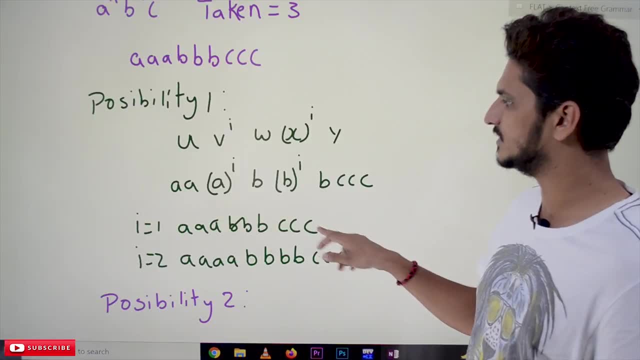 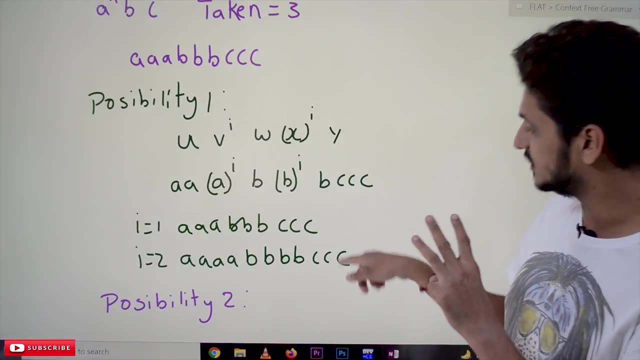 for I is equal to one. what we will get? a, a, B, BB, C, C, C for I is equal to 2 a, a, 4 a, followed by 4 B's, but there are no C's, 3 C's, which is this string is not present. 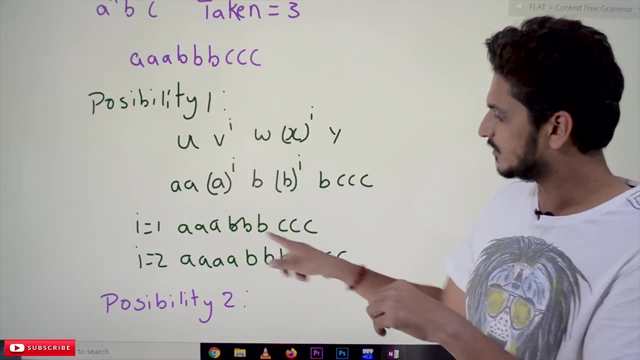 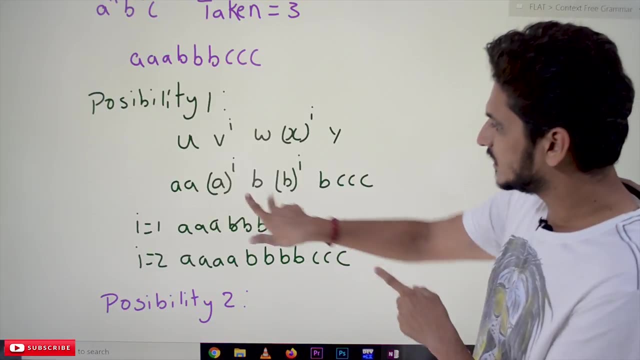 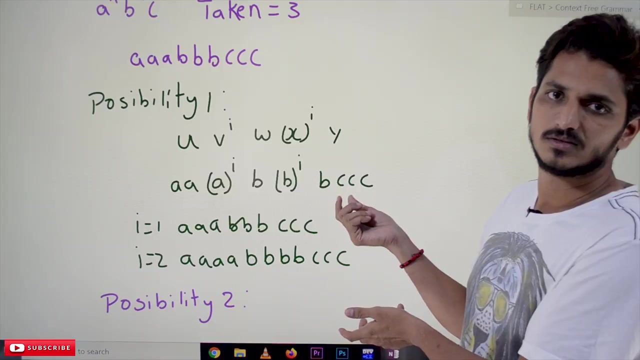 in our language is followed by equal number of B's, followed by equal number of C's. that is what our language is: a power n, b power n, C power n. if you take these two variables and pump, we are going to pump a, B, but we are not able to pump C. so this possibility, in this possibility, we are 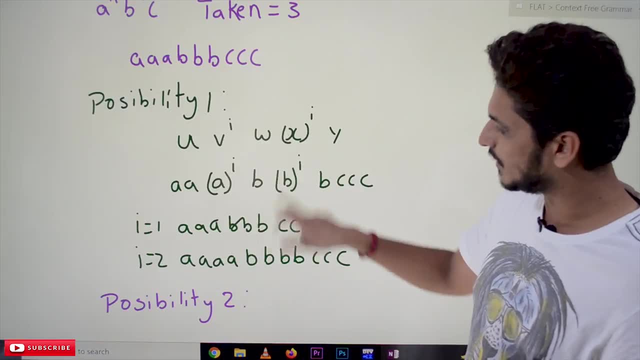 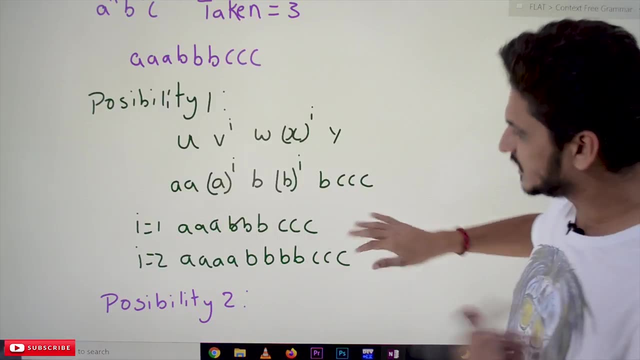 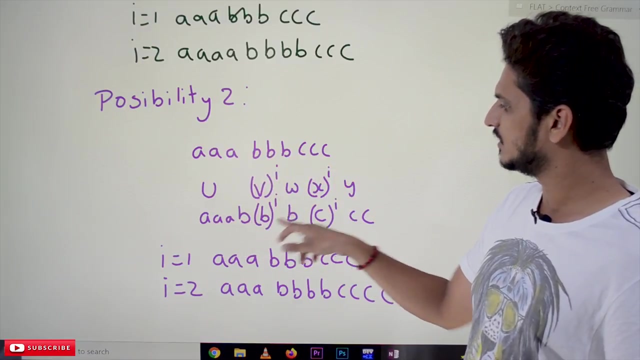 not getting a the language, the strings that are, if he keeps on pumping, we are not getting the strings that are present in this language, present in the language: a power and b power and c power, n, like the. take another possibility. we're taking one more possibility: a, a, b, b, b, c, c, c. you as a, a, b, b, s, b, w, s, b, x, s, c, under. 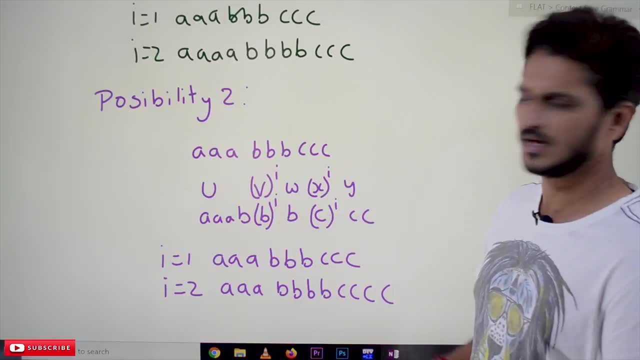 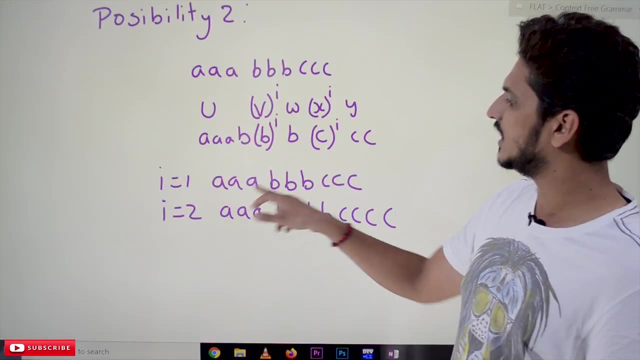 a, y, s, c, c. if he keeps on pumping v and X, this B C is going to pump. we are missing a. that is how. so I is equal to 1 a a, a, b, b, b, c, c, c. i is equal to 2 a a a. 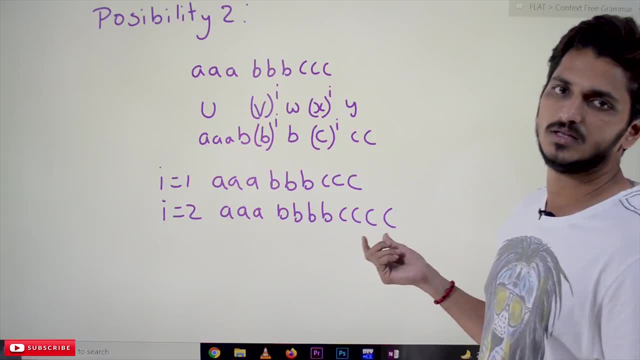 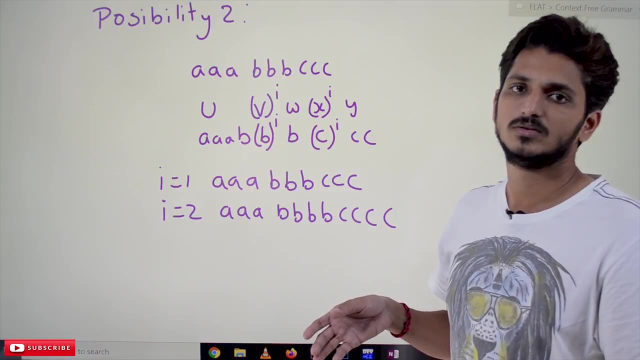 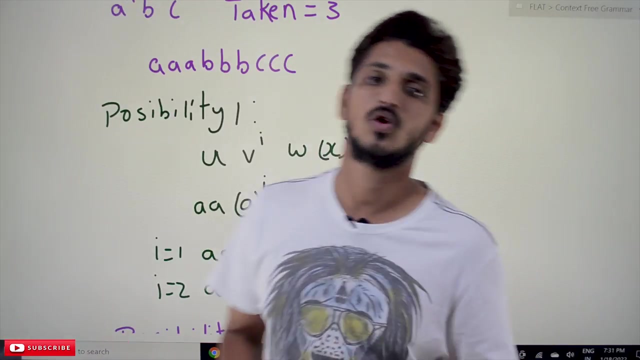 b, b, b, b, c, c, c, c. so in this possibility also, we are not going to generate the strings that are present in the language. so if you show that all the possibilities are not going to generate, then we can say that the the given language is not a context-free language. this is how we will show that we will use pumping. 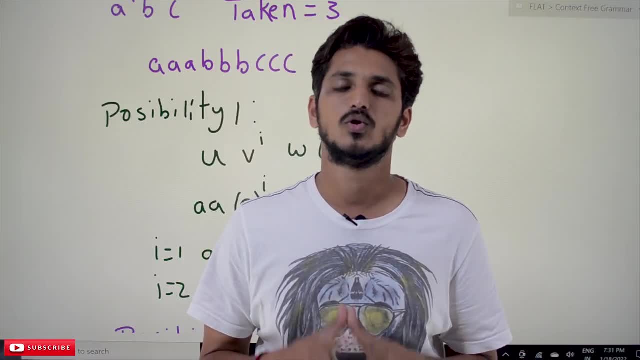 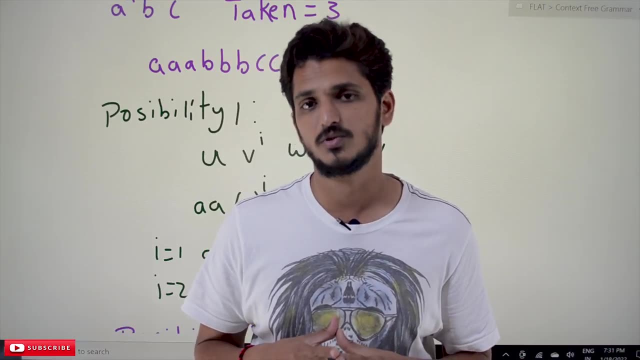 lemma to show that the given language is not a context-free language. hope you understand the concept. if you have any questions regarding the concept, please post your questions in the comment section below. thanks for watching. if you haven't subscribed to our channel, please subscribe to our channel and press bell icon for the latest updates. thank you. you.